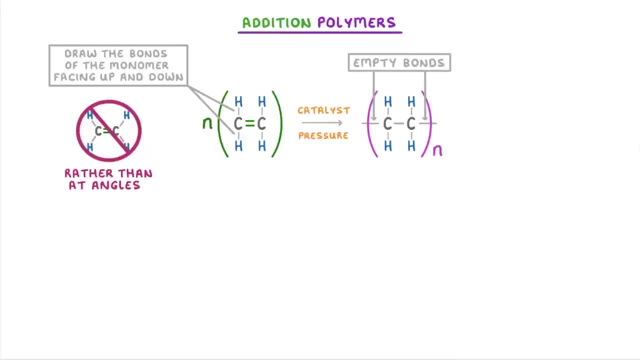 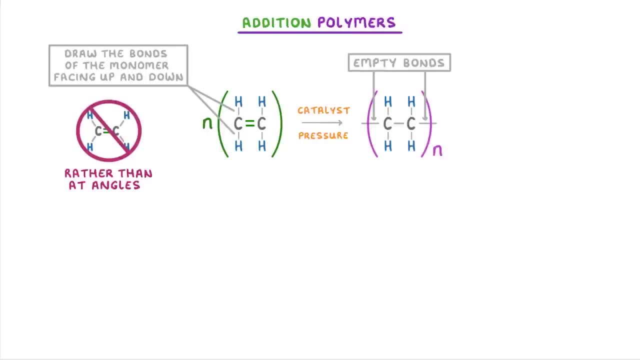 that go through the brackets. The other important feature are the n's, which represent how many of the monomers and thus how many repeating units there are in the reaction. For example, if n was 10, then that would mean that there were 10 ethene molecules on the left. 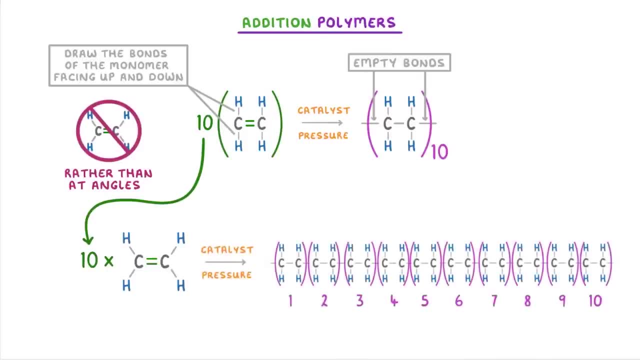 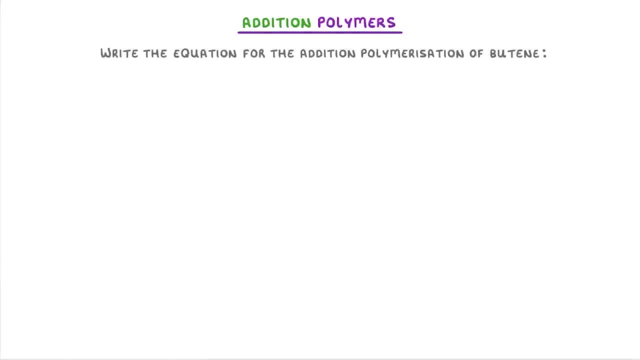 and so the polymer would be 10 repeat units long. To put all of this together, let's try and write an equation for the addition polymerization of butene, which is this: 4-carbon alkene. The first thing we need to do is redraw the butene. 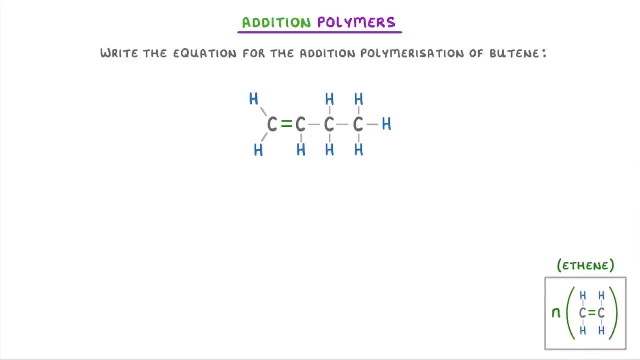 so that it's in the same format as this diagram of ethene that we just saw. To start, we need to identify the double bond which is here between the first two carbons. Let's do that. Next, we need to arrange all of these atoms as separate groups. 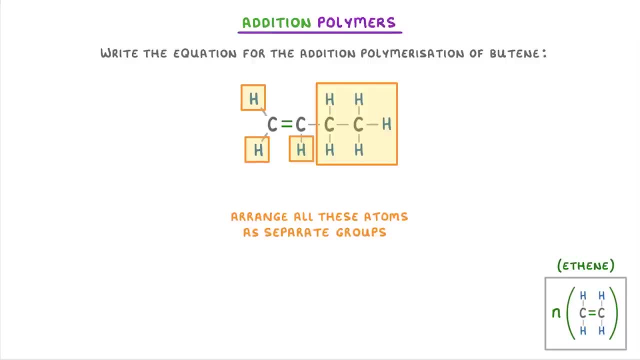 because they're the groups attached to the carbons of our carbon-carbon double bond And if we look back at our ethene example, we need to place them directly above and directly below the two double bonded carbons. To do this for butene, let's start with our two double bonded carbons. 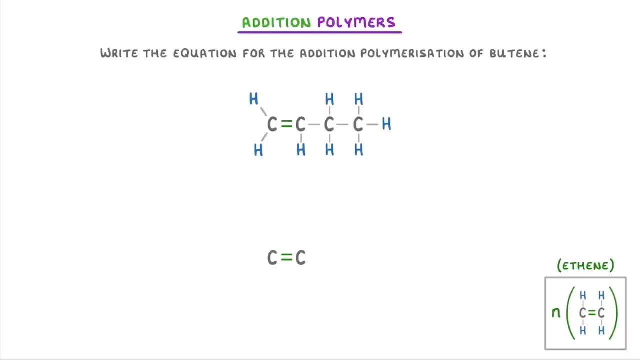 and then we'll rearrange each of the separate groups one by one So that it's easy to follow along with what's happening. This first hydrogen needs to change from being shown sticking out at an angle to being shown, like this, pointing straight up from the carbon. 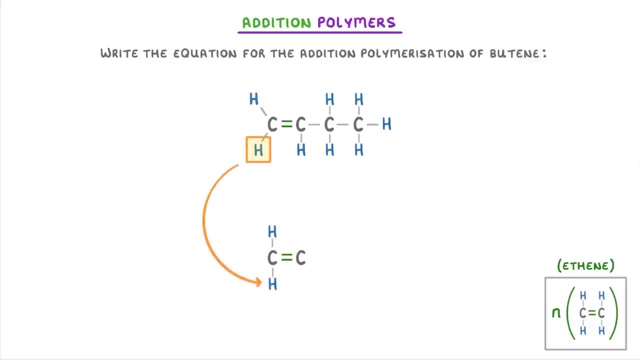 And we do exactly the same thing for this hydrogen, so that it points straight down rather than sticking out at an angle. Then this hydrogen over here is already pointing straight down, so we just redraw it exactly the same way. Finally, for this big group. 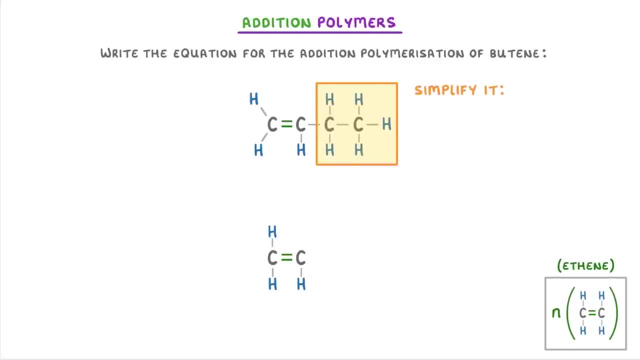 on the right, we use a little trick and simplify it before moving it about. To do this, we just count up all the carbons and hydrogens and write them out in shorthand. So because there are two carbons and five hydrogens, we write this group as C2H5. 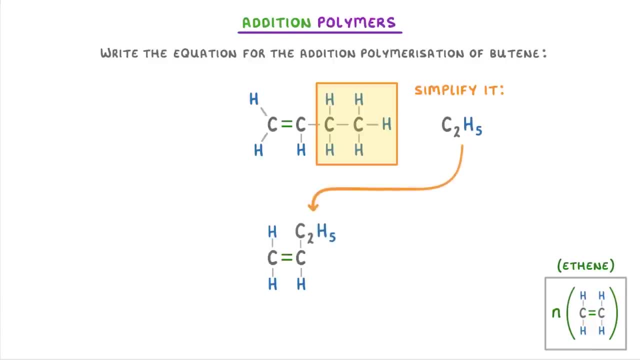 And then we just do exactly the same thing as before and rewrite the group so that it's directly above our double bonded carbon. One thing to be aware of is that when we do this, we don't want our double bonded carbon to be the same as the first group. 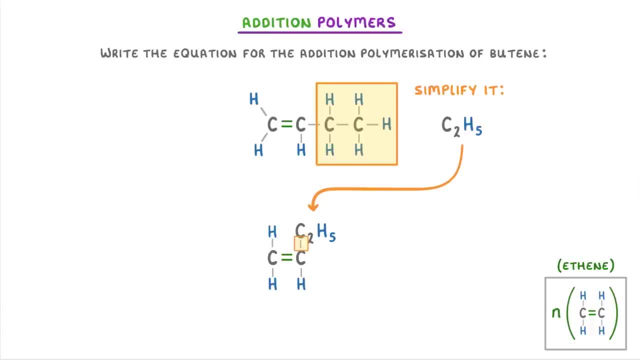 It's important that this bond is drawn going from carbon to carbon rather than to the H5 part. Now that it's drawn in the right format, we can add the brackets and put the n in front of it. Next, we can draw our reaction arrow and then draw the other side of the equation. 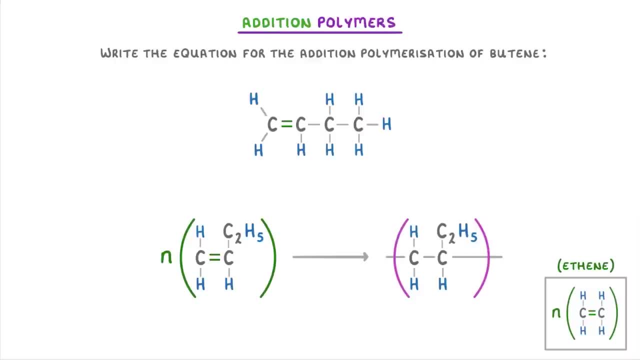 that shows the repeating unit. We draw pretty much exactly the same thing, but notice that we've taken out the double bond and instead put the carbon's bonds out to the sides extending through the brackets. And remember, for a repeating unit the n goes here on the bottom right, just outside the brackets. 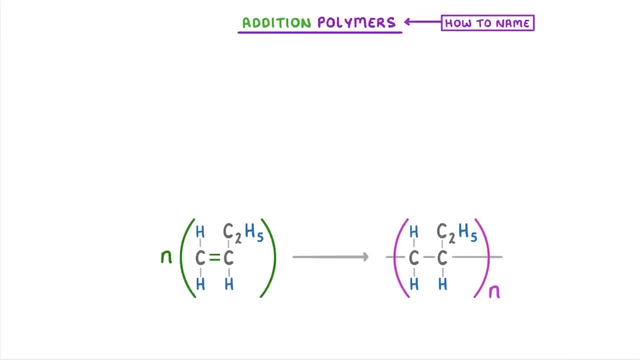 The last thing we need to cover is how to name the polymers, which is actually really easy, because all we have to do is put the word poly in front of the monomers and put the monomers name in brackets. So in our example here, where we're drawing the polymer of butene, 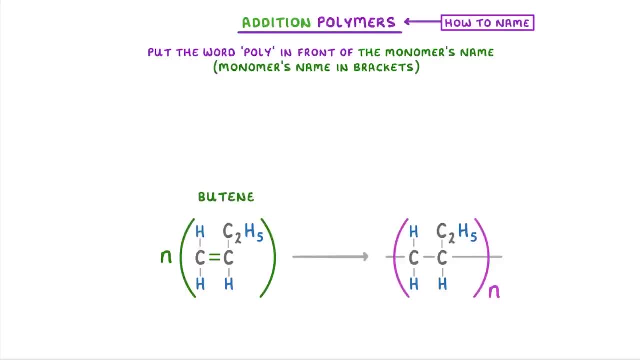 the monomer is butene and therefore the polymer is called polybutene. Or if we go back to the first example we did, the polymer would be called polyethene. Or if we had this monomer which is called chloroethene. 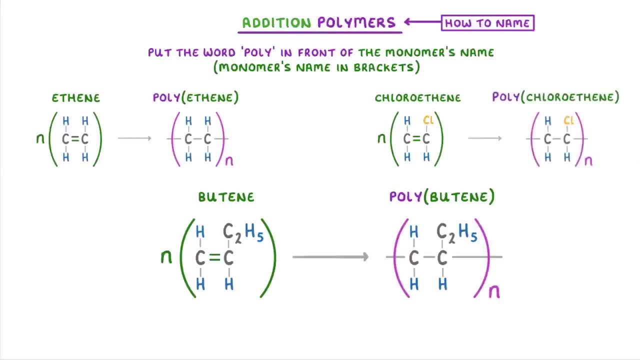 we'd make the polymer polychloroethene. The very last thing we need to mention is that these addition polymerization reactions require high pressures and a catalyst to work, So you might sometimes see pressure and catalyst written on the reaction arrow. You don't have to put this on the arrow yourself, but you might be asked for these two conditions. 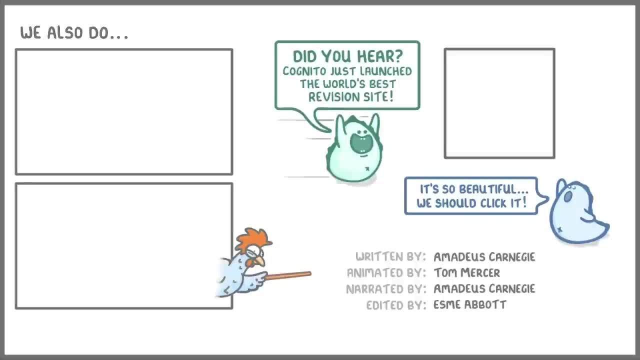 They're exactly the same, but they're possible. Anyway, that's everything for this video, so I hope that all made some sense and cheers for making it through to the end.